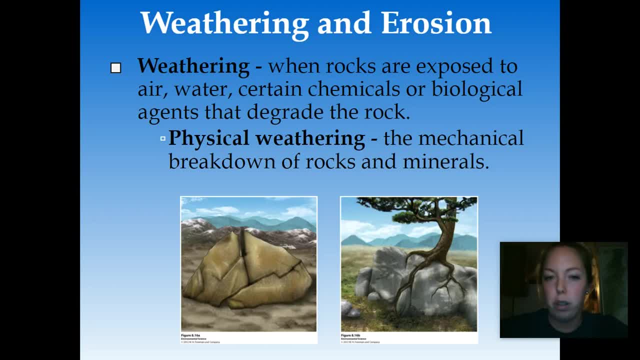 sediments and that concept of you know, the rock cycle, recycling, Okay. so let's talk about weathering for a second right. Weathering is a process that goes down when the rock is exposed to air, water, certain chemical compounds, or it could be biological agents, Okay, like plant roots. 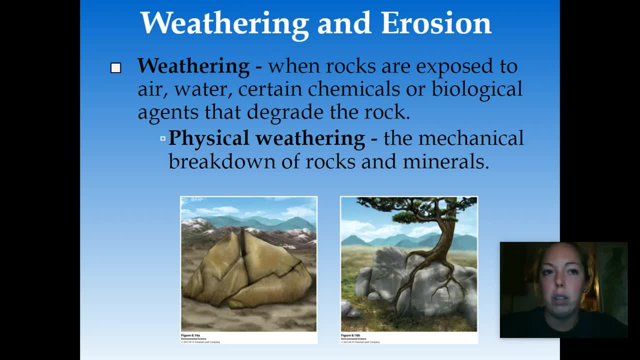 lichens. we'll talk about that when we talk about ecological succession, burrowing animals, etc. all sorts of stuff like that. So there are two different types of weathering that we're going to talk about, but the first one's called physical weathering. Okay, so you can see it right here. yeah, 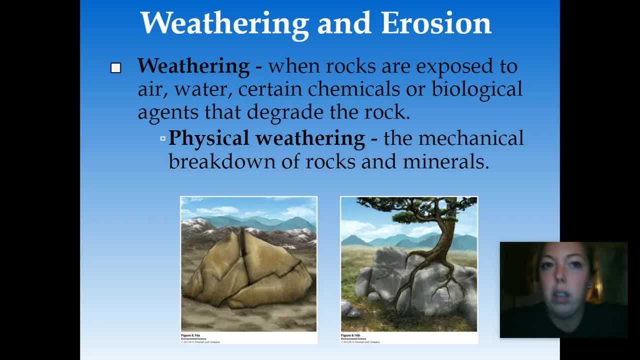 but basically, when we talk about physical weathering, we're talking about the type of weathering that has to do with the mechanical breakdown of rocks and minerals. Okay, so the physical breakdown: this can be from water, wind or things like seasonal freeze thaw cycles. So 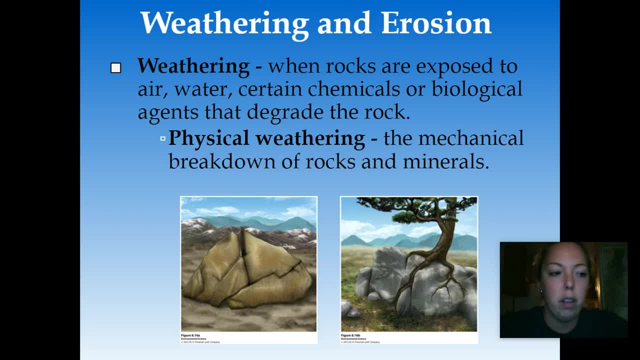 for example, you guys are from Texas so you might not know, but if you ever lived up north, where it gets really cold in the winter, the water freezes and what happens is the water gets down into the cracks of the road and when it freezes it expands right, and so we have a lot more damage. 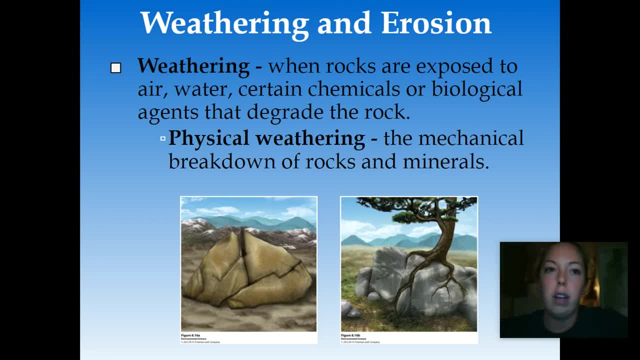 up north to the roads and stuff, because of these seasonal cycles and stuff like that. So that's an example of physical weathering. Okay, like I said before, another way physical weathering can happen is from biological agents. so a really good example of this would be plant roots. Plant roots can work their way into small cracks in the 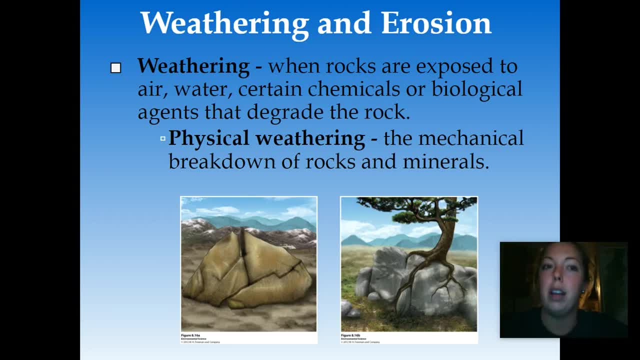 sidewalk or wherever it may be, like the foundation of your house, and they can slowly pry the cement apart. okay, So that's really bad right. But basically, no matter what way physical weathering happens, it's going to expose more surface area. When more surface area is exposed, 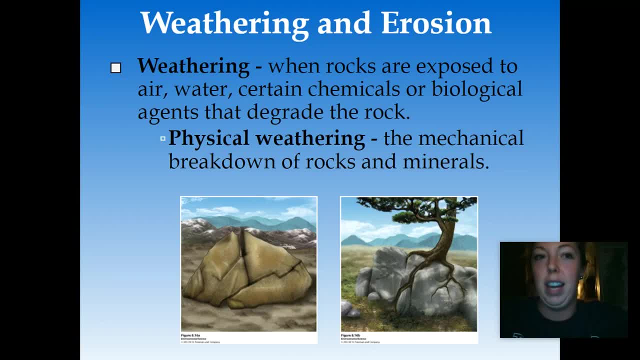 the rocks are more vulnerable to even more weathering. okay, So basically, it allows more surface area for chemical weathering to later act on. all right, So it would be safe to say that physical weathering increases the rate of chemical weathering. okay, So let's talk about that next. 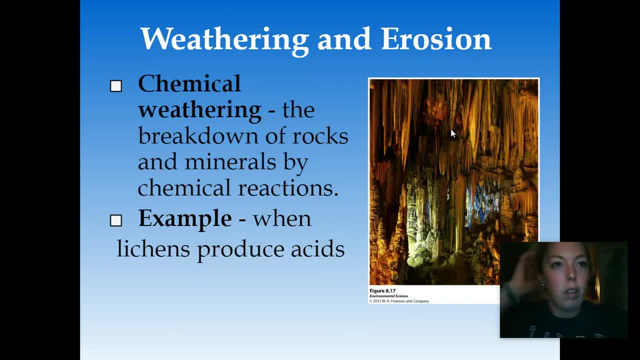 all right. So chemical weathering: okay, This is the second type of weathering. all right, It's a lot different from physical weathering, because this is the breakdown of rocks and minerals by chemical reaction. specific, This could be the dissolving of chemical elements from the rocks. 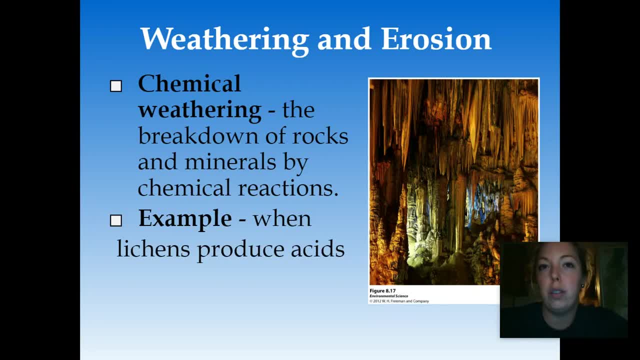 or both, but basically it releases essential nutrients from the rocks and it makes them available for use by plants And other organisms that might use those nutrients. So if you guys can think back to chemistry, you learned about solutions right, And if they are basic or acidic, Depending on 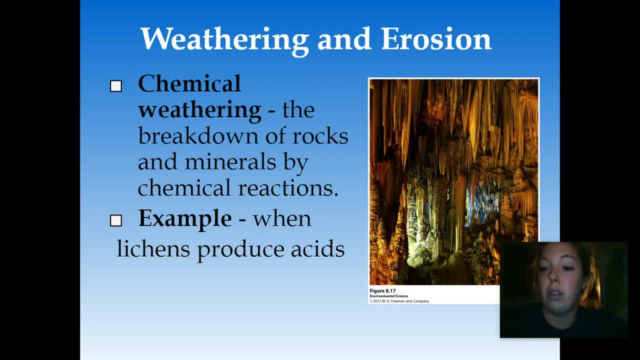 the starting chemical composition of a rock and the pH of the water that comes in contact with the rock. there could be hundreds and hundreds of different chemical reactions that take place, okay. So, for example- and we'll talk about this a lot when we talk about climate change- 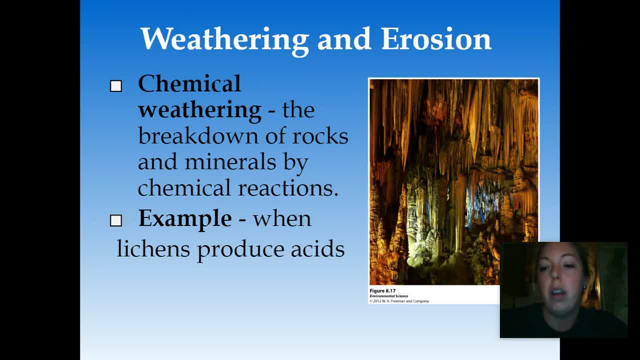 carbon dioxide in the atmosphere is able to dissolve in water, right. So when that happens, it creates a weak solution of carbonic acid. okay, So when waters containing that carbonic acid flow into limestone-rich geological regions, they can dissolve the limestone, because the limestone is composed of calcium carbonate and they can make really 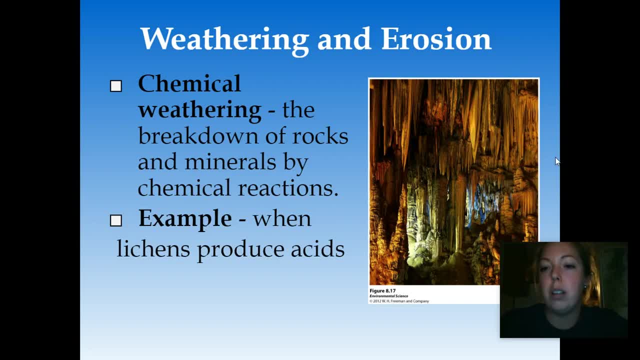 really cool cave systems like the one right here. okay, We're going to talk about this during climate change a lot. when we talk about seashells, Yeah, so the seashells of organisms in the ocean are actually dissolving because the acidity of the 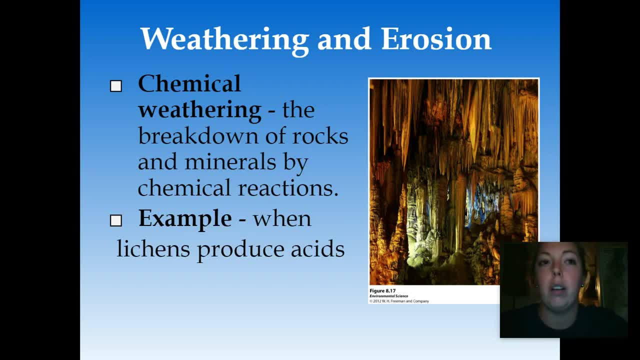 ocean is increasing, okay, So it's really really kind of crazy. Anyway, some chemical weathering is because of human activities, right? So an example of this could be sulfur emitted in the atmosphere as a result of fossil fuel combustion, right, When that sulfur is emitted into the. 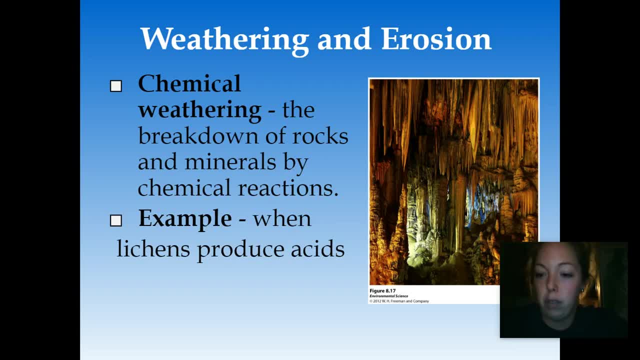 atmosphere. it combines with oxygen and it forms something we call sulfur dioxide. okay, Basically, the sulfur dioxide reacts with water vapor in the atmosphere and it forms something called sulfuric acid- all right- which then causes acid precipitation or acid rain. You guys have probably heard of that before. We're going to talk all about acid rain during our 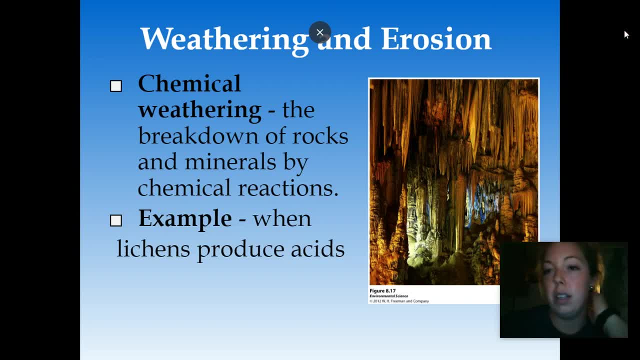 pollution unit okay. But basically this does a real job destroying statues. It can destroy gravestone, gravestones, limestone, marble, anything like that, okay. And when that acid rain falls on soil as well, it can cause chemical. 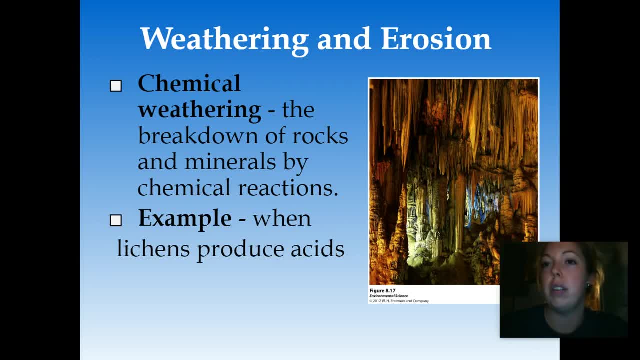 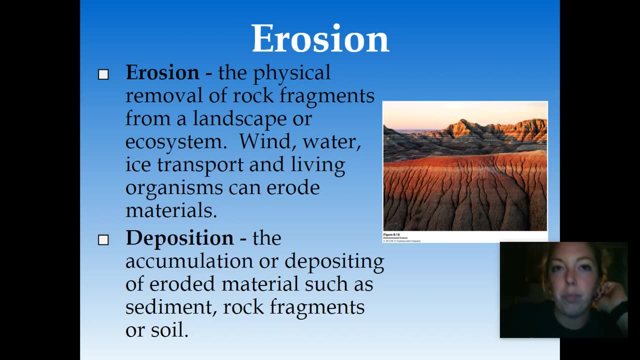 weathering of certain minerals in the soil, which releases elements that can be taken up by plants or leached from the soil into groundwater streams and stuff like that. So it's really bad news bears. okay, Let's talk about another really important thing real quick before we get into soil stuff. all right, So erosion. I often see that a lot of students get erosion and weathering. 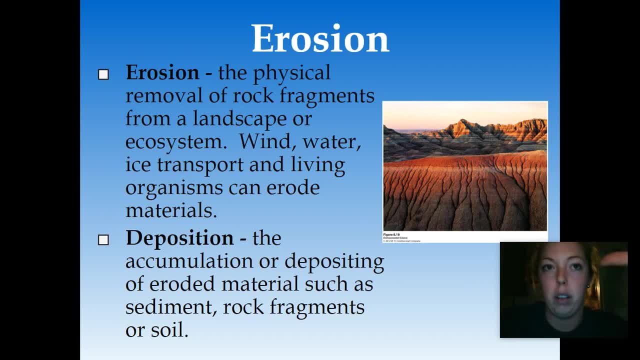 confused, so I'm hoping that this will make sense and they will be straight in your brain, all right. Basically, though, we just talked about how physical and chemical weathering results in the breakdown and chemical alteration of rock. okay, Erosion is a little different, all right. Erosion is simply the physical removal of that rock from a landscape or an ecosystem. 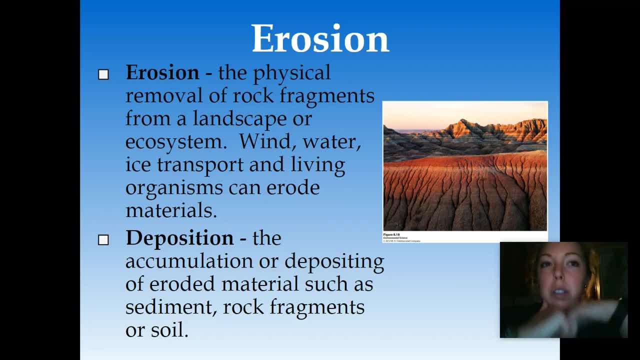 ecosystem. Okay, so erosion is usually the result of two different mechanisms that we're going to talk about. Okay, all sorts of things like wind, water, ice- those things can transport soil. Oh, look who it is. It's my puppy, It's Kiba. and Mr Morales He said: hi Kiba, Isn't he cute. 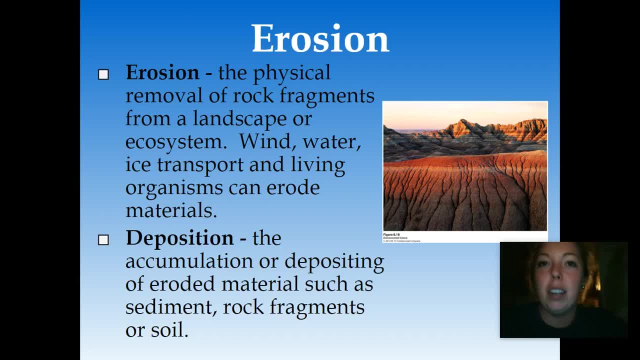 Um, what was I saying? Okay, yeah, wind, water, ice, stuff like that. It transports soil and other materials downhill right via gravity, Makes sense. So living organisms, like things that burrow under the soil and live in the soil, also can cause erosion, But basically after eroded. 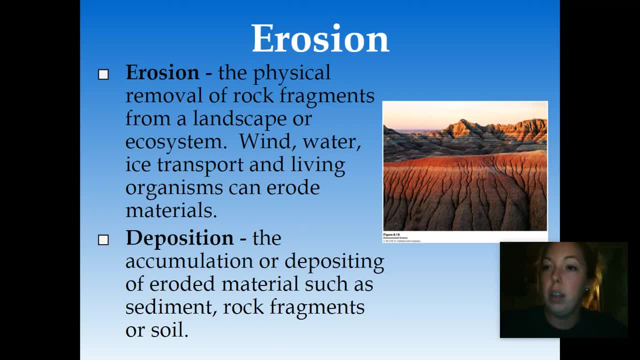 materials have traveled a certain distance from the source, it accumulates. right, We call this deposition, All right. so that's your second vocab word, right here? All right, deposition. Deposition is the accumulation or depositing of eroded materials such as sediment. 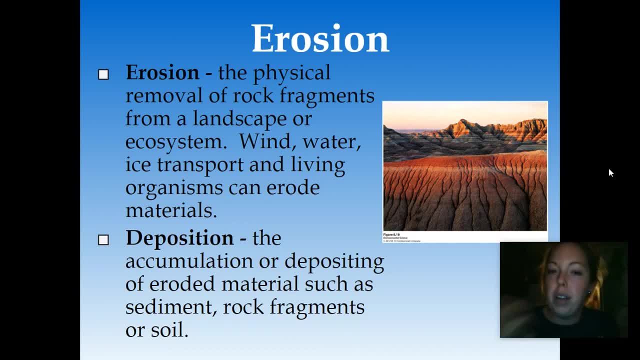 rock fragments or soil. Okay, and when you guys learned about the rock cycle, you learned that sedimentary rocks are simply sediments deposited over and over and over in layers. Okay, so this is what you would see here. You can kind of see the lines and the rocks there. 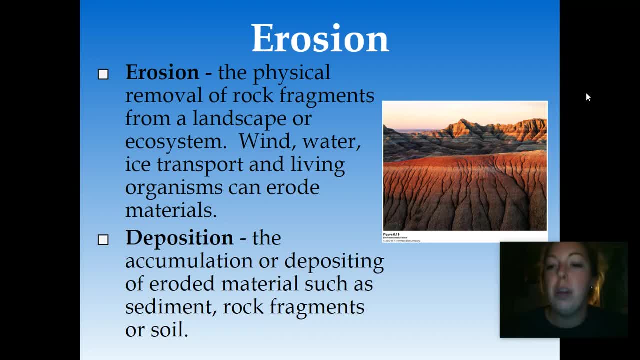 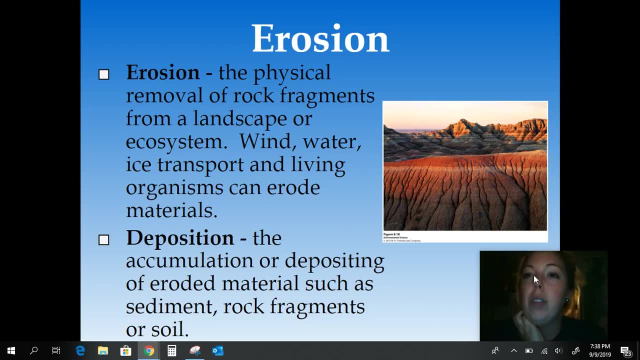 That's what it looks like once it's deposited. So the thing with erosion is that it's always been a really natural thing, right? But in lots of different places, the way that we use land can really really increase the rate of erosion, which is a big 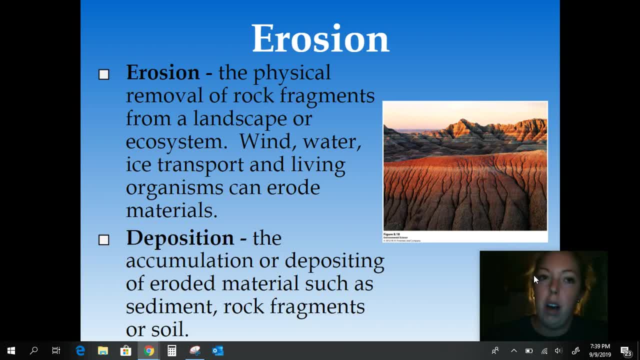 big problem. Okay, so depending on our methods, you know, if we are deforesting areas, we're overgrazing cattle or something like that. If we have unmanaged construction activity in a certain area that can accelerate erosion problems, All right, that's not the only bad. 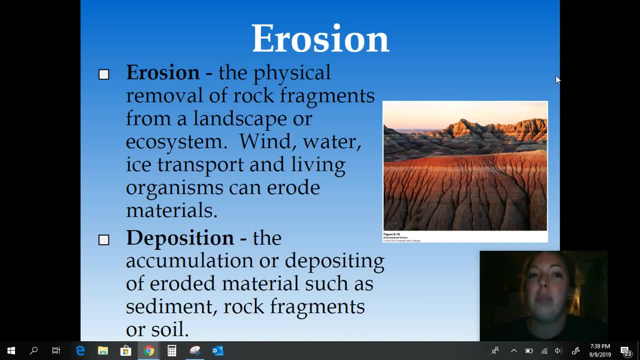 part, though, because usually erosion is going to lead to deposition of the eroded rocks somewhere else, Okay, which could cause even worse environmental problems. All right, we're going to talk way more about that when we get into our land use unit, So keep that in your brain and we'll talk about it. 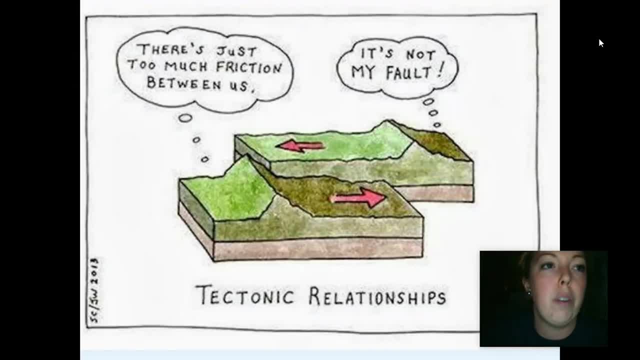 here in a little bit. Here's a little joke for you, if you want to see it. There's just too much friction between us, Isn't that funny? It's not my fault. It's not my fault. Tectonic relationships. 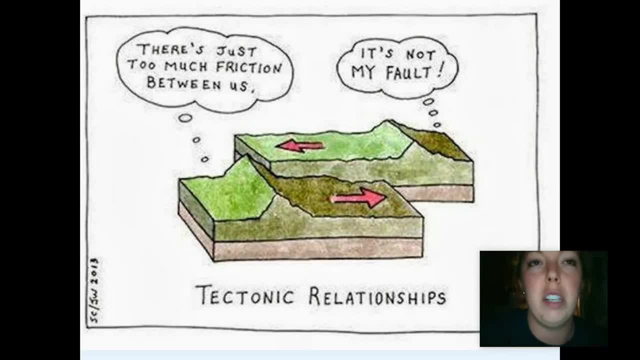 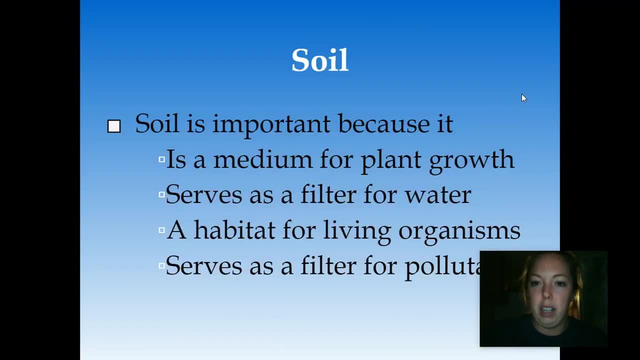 As a geologist, I find that hilarious. Mr Morales thinks it's funny, so you guys better. Okay, let's see. Now let's talk about the good stuff. Remember, today in class we were talking about soil and you guys said it was just called dirt. No, it's actually really cool. It has a whole 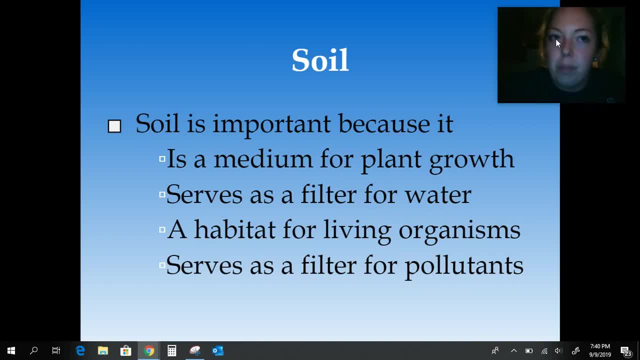 bunch of cool stuff in it, So this is why it's important. Let me tell you All right. we talked about during the first week of school how soil is one of the most important resources that we have And you know it's critical that we take care of it If we don't have healthy soil. 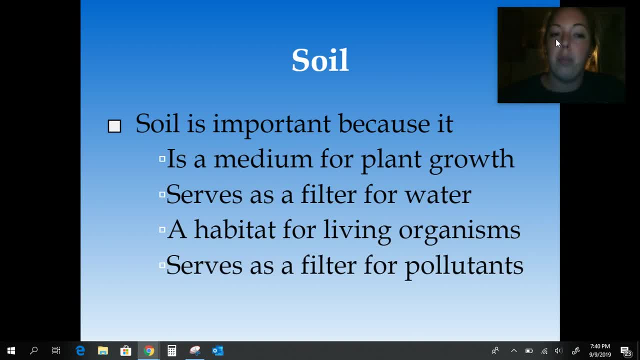 we don't have plants to create oxygen that we breathe. We also don't have plants to grow that we eat or that we eat. So we don't have plants to create oxygen that we breathe. We also don't have plants to create oxygen that we feed to other things that we eat. Okay, for those of you, meat. 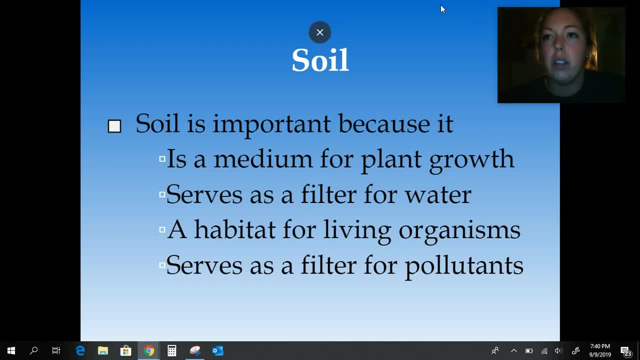 eaters out there. Let's talk about this. It's essentially the third part of the geologic cycle and we call it soil formation. Soil is a mix of geologic and organic components. I know when you guys think of soil you just think of dirt. It's the stuff in the ground that nobody 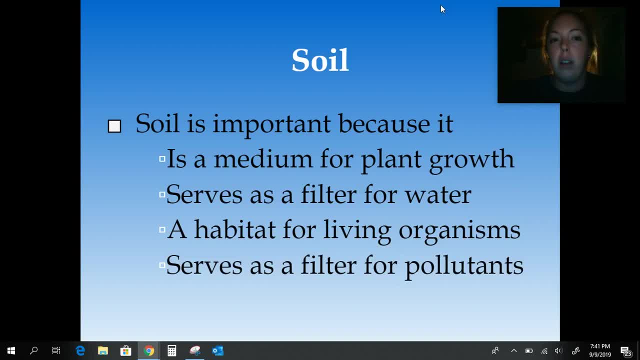 cares about right. So there are a whole bunch of reasons why soil is so amazing, And these are some of the reasons listed right here. Okay, so it's obviously a medium for plant growth. Okay, it also provides water, As water moves through the atmospheres into rivers, streams, groundwater. 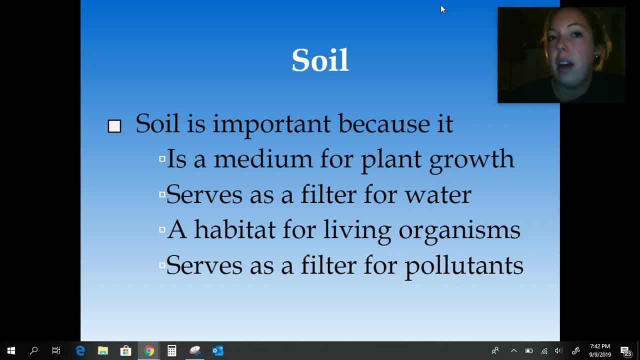 stuff like that. Soil provides habitat for a wide variety of living organisms. It can include things like bacteria, algae, fungus, fungi, I guess you could say all the way up to insects and other animals. Okay, so that's one of the things about soil that you guys probably never, ever think about. 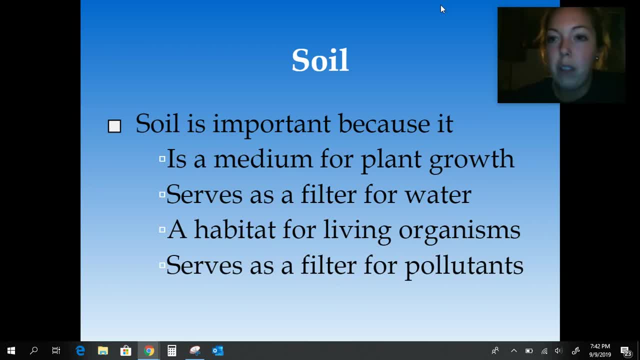 right, There's so much biodiversity in soil. Okay, the biodiversity in our soil is really, really important because they recycle organic matter. Okay, so these organisms that live in the soil- they're able to take dead stuff, So it could be dead. 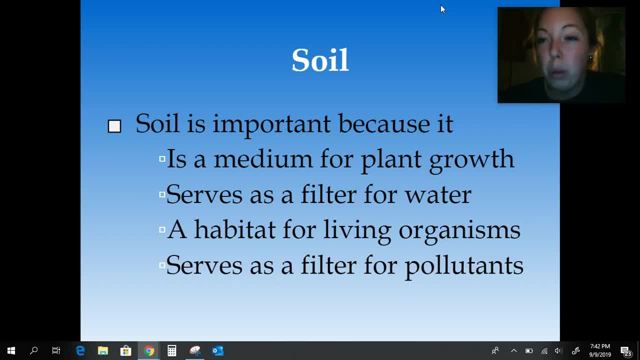 animals, whatever it may be, or their waste. So I'm talking poop, right, the poop of animals, and they can break it down to use as an energy source. This is really, really awesome. But basically they do this by breaking down organic detritus and they release mineral nutrients and 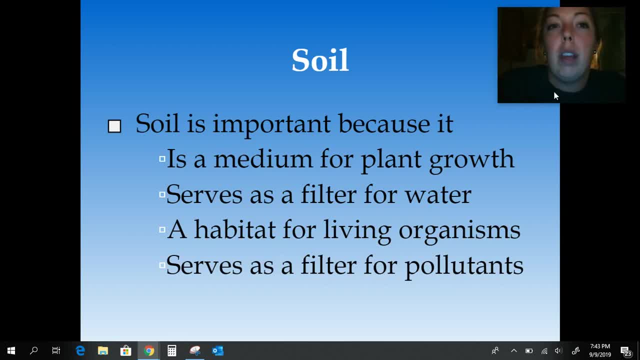 other materials that benefit plants to the plant. So soil and all these little guys within it also are really, really important. Okay, so we're going to talk a lot more about that. Okay, so here's a little diagram that's essentially showing all the reasons why soil is important, like what I just 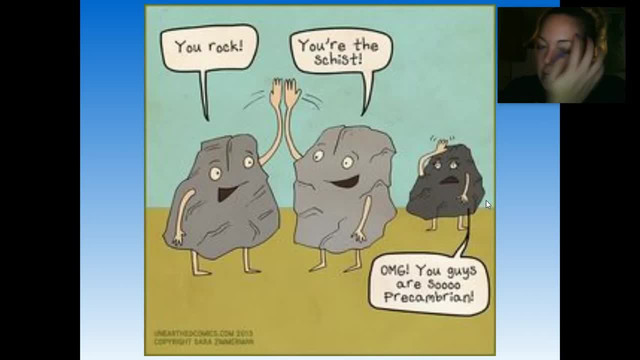 said: Here's another one. Let's see. Oh yeah, this is funny. Ha ha ha, you rock. You're the schist. Oh my god, you guys are so pre-Cambrian. This is a type of rock, If you guys don't know. 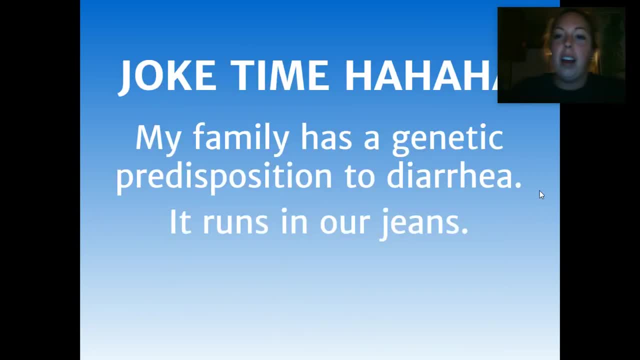 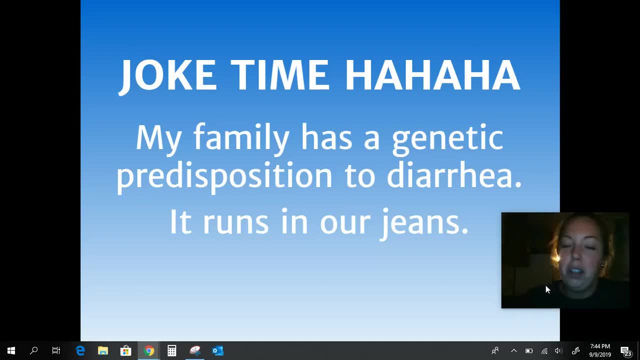 you guys didn't do your lab the other day. Okay, oh, joke time. Let's see what is it. Oh my gosh, this one's pretty rough, but I thought I'd put it on here anyway. So the joke is: my family has a. 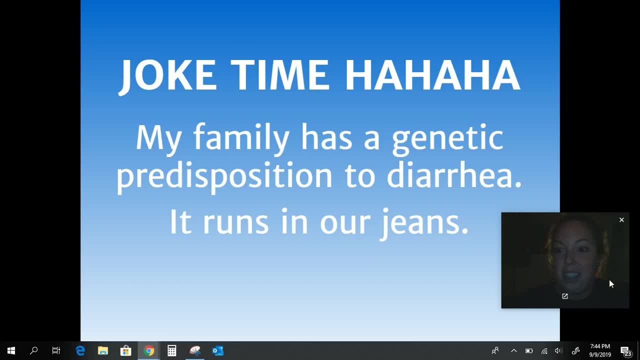 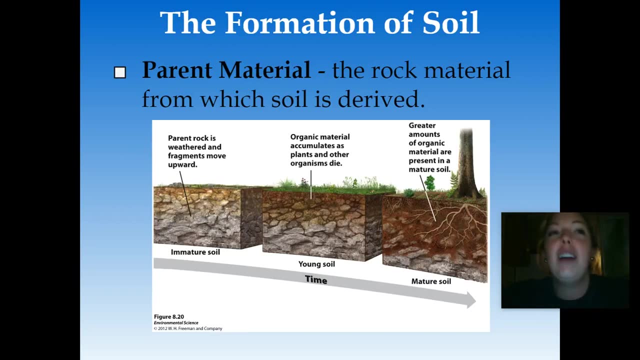 genetic predisposition to diarrhea. It runs in our genes. All right, let's go to the next one. Okay, so let's talk about this. Oh, I have no life. All right, so the formation of soil. Oh, we're getting into the good stuff, Aren't you guys excited? 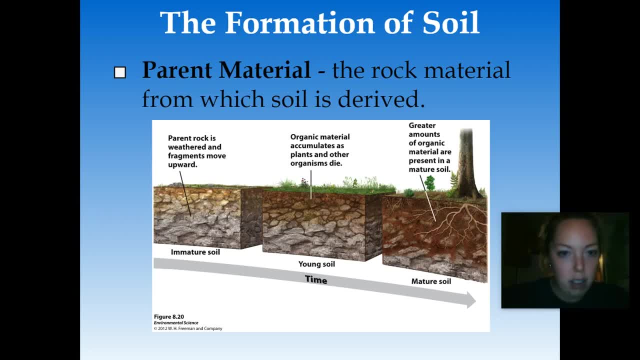 All right. so, like we talked about in class weeks and weeks ago, it takes hundreds and hundreds and hundreds of years for only a little itsy bitsy bit of soil to form. Okay, so we're talking like 500 years for about an inch of soil to form, but you can completely destroy that inch of soil in one 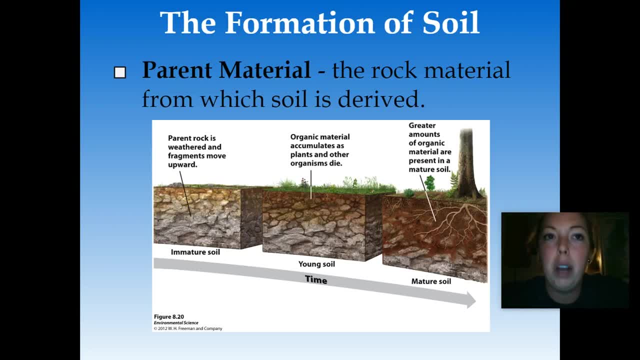 bad planting season. Okay, so that's pretty messed up, But anyway, this is what we need to talk about right now: The fact that soil is the result of physical and chemical weathering of rocks, right, And the gradual accumulation of detritus from the biosphere. Okay, So we can determine the 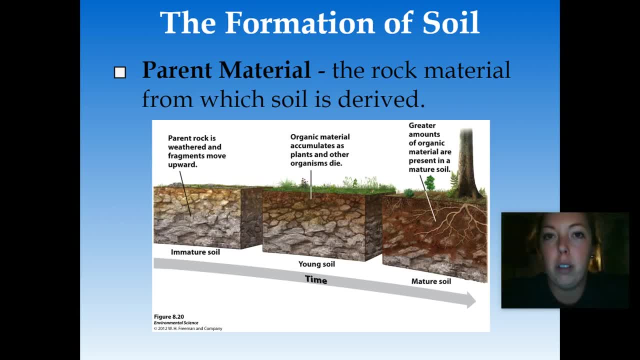 specific properties of a soil if we know a few different things about it. Okay, so some of the things that we have to know in order to do that are the parent rock type, we have to know the amount of time during which it's been forming, And we have to know the biotic and abiotic. 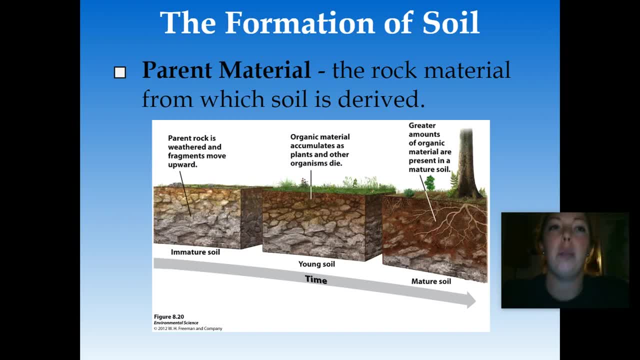 components associated with the soil. Okay, so the processes that form soil work. they're going to be in two directions simultaneously at the same time. So we've got the breakdown of rocks and primary minerals by weathering. that's going to provide the raw material for soil from. 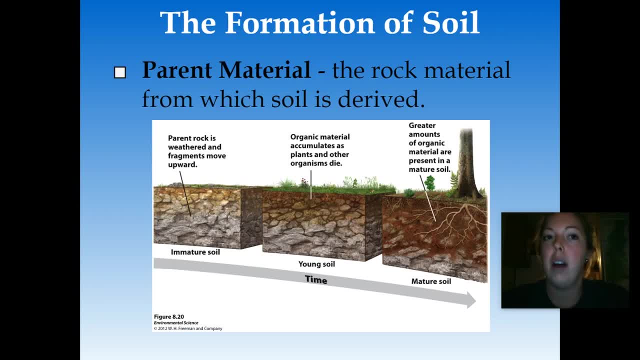 below, from the earth, right You also have. the second thing is the deposition of organic matter from organisms, So it could be dying organisms not dying, but dead organisms and also their poop, their waste, right That's contributing to soil formation from above. Okay, those two things. 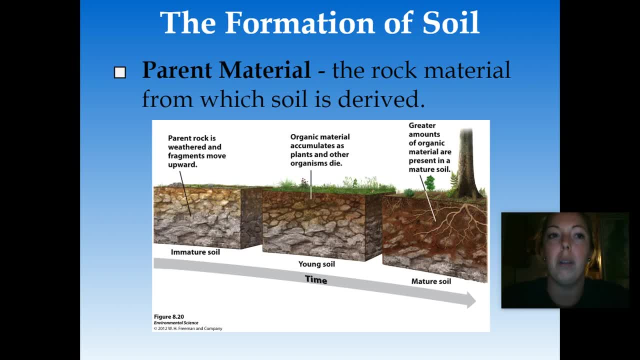 combine Are going to determine all sorts of things about the soil. Okay, So what we normally think of as soil is a mix of these mineral and organic components. Okay, a poorly developed or young soil which you guys can see over here where it says immature or young, It's a soil that has way. 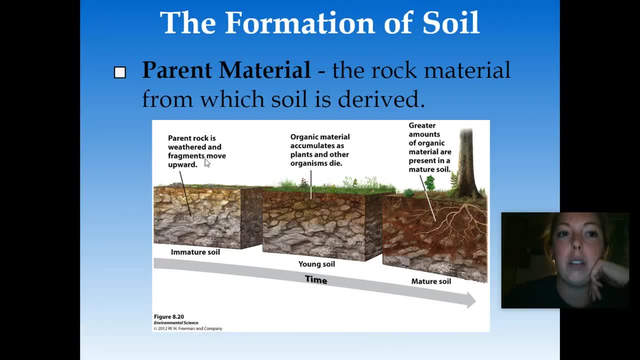 way, way less organic matter and fewer nutrients. compared to that which would be a mature soil, This one is going to be more developed. it has more nutrients. it has more organic matter, all sorts of good stuff in the soil. This would be a good soil. 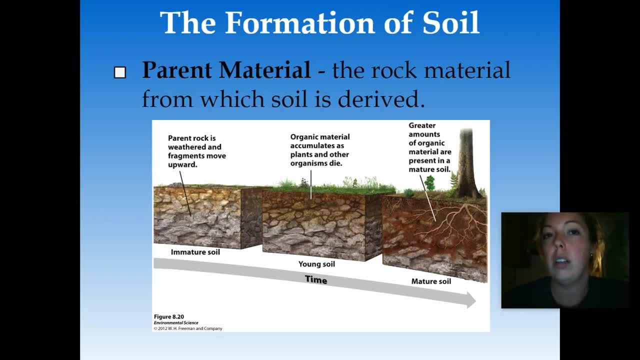 compared to this soil over here, right, Very old soils could be nutrient poor because over time plants are removing many of the essential nutrients from the soil right. They have to use them so they can grow big and strong, Or those nutrients could be washed away by the water. 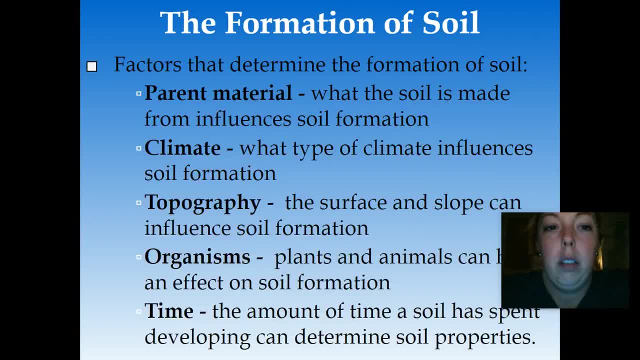 depending on where your soil is. Here's a slide which is listing the five factors that determine the properties of soils. Okay, I'm not going to go through all of them, but I'm going to go through the five factors that determine the properties of soils. Okay, I'm not going to go through all of them. 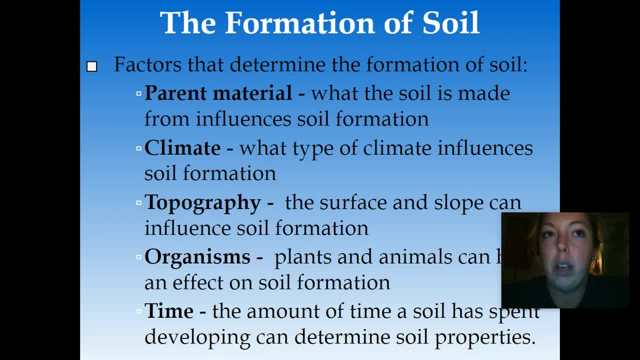 Okay, I'm not going to go through all of them, but I'm going to go through all of them. I'm not going to talk about these too much, But make sure you read through each one in your book to make sure that you get the gist of it. Let me move my face over here so that you can see. 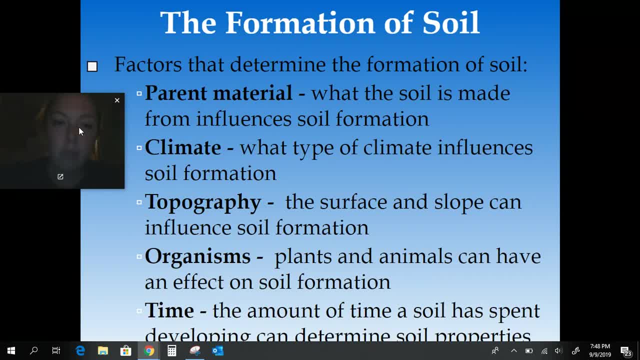 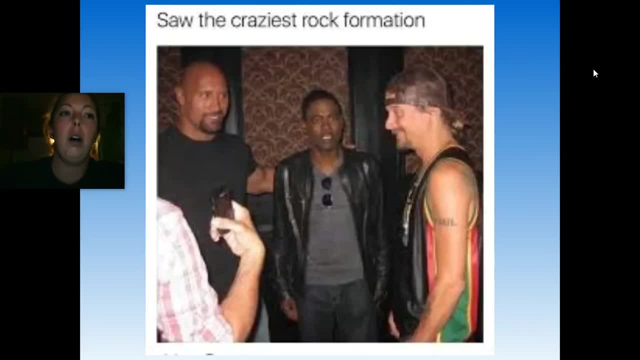 everything. Okay, Yeah, be familiar with these five different concepts. Okay, I'm going to save that for you guys to go over it in your book. Oh, this is funny. Look how funny this is. Okay, you don't see it? Oh, I already showed Mr Morales He thinks it's funny. It's the craziest rock for. 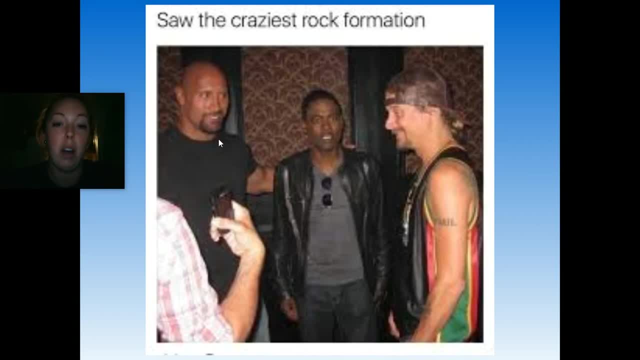 formation. And if you guys are too young, it's the rock, It's Chris Rock and it's Kid Rock. No one knows two of those three people. No, and the picture is really blurry. But okay, let's talk about soil horizons. 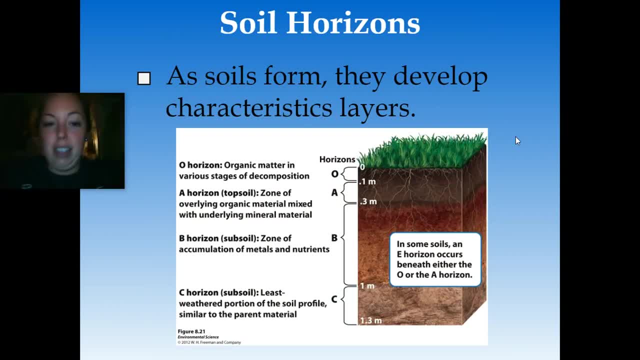 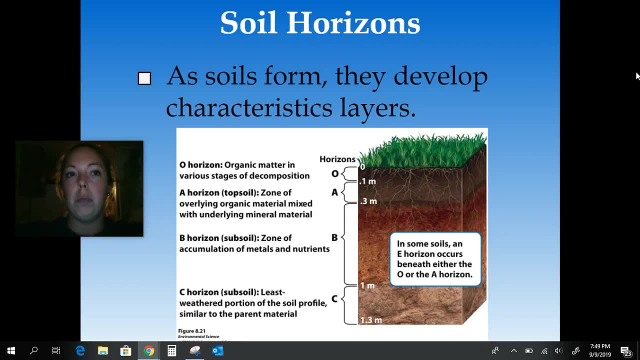 Okay, so this is another thing that you guys need to know. So, depending on the location and all of these factors that influence the soil, these soils can serve different properties for us as humans. right? Some of those soils are really good for growing crops. 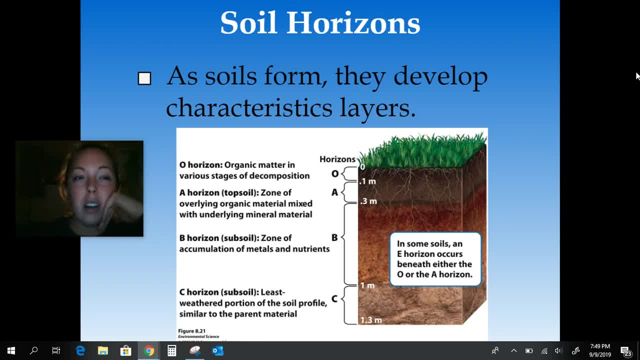 some of them are good for building a house, like a foundation on right and stuff like that. So we're going to talk about that and the differences between them. So, in order to understand and classify our soil types, which you guys can see here, we have to understand soil horizons and 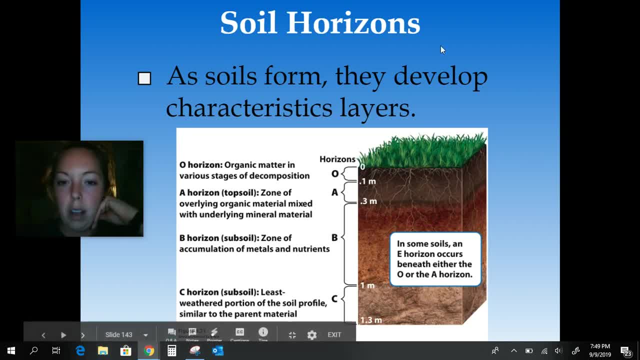 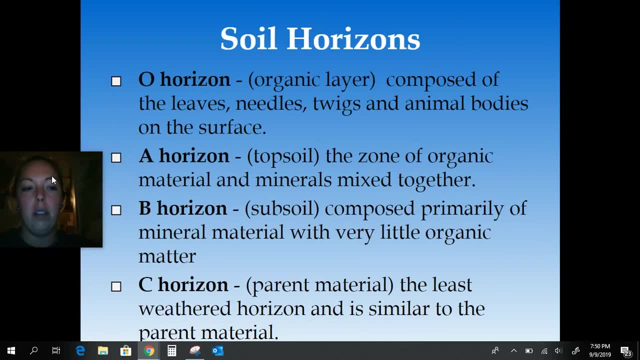 soil properties. Okay, so I'm going to go to the next slide and try to get this image here in your head, But these are the different soil horizons that we have to know about. All right, I'm sorry you guys are looking at my double chin this whole time. 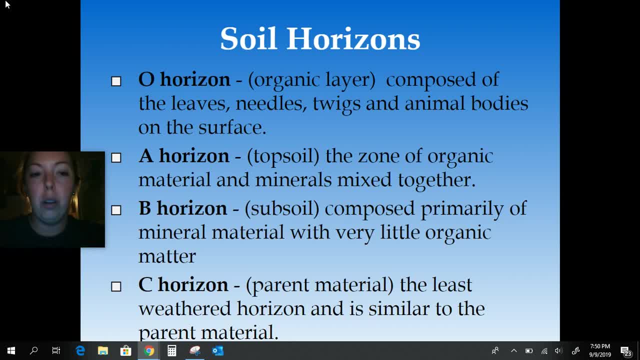 Okay, so for soil horizons: basically, as soils form, they have different characteristic horizons. Okay, that basically just means layers. But you can see in the picture, you know, on the other slide right here, if I go back right here, these different layers are forming okay. 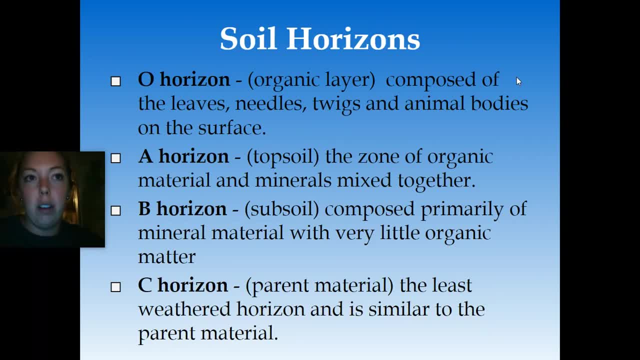 But the composition of these horizons or these layers depends mostly on a bunch of different things like climate, the value of the soil and so on and so forth. So if I go back here I can see the vegetation that's present in the area and also the parent material that the soil has come. 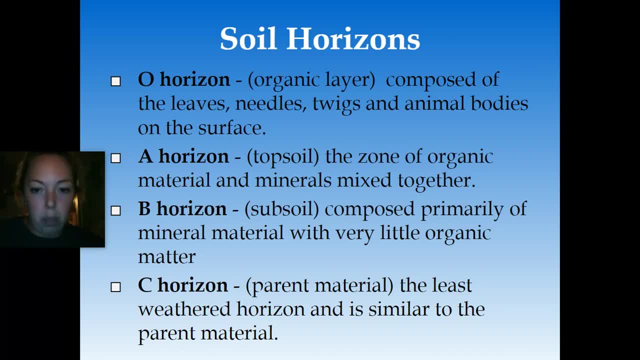 from Okay, And they're all different for all soils everywhere on the planet. That's why you can see, when we're doing our lab in class, those eight different bags or samples that I have for you. they all look different, they feel different, they have different textures. right, They have. 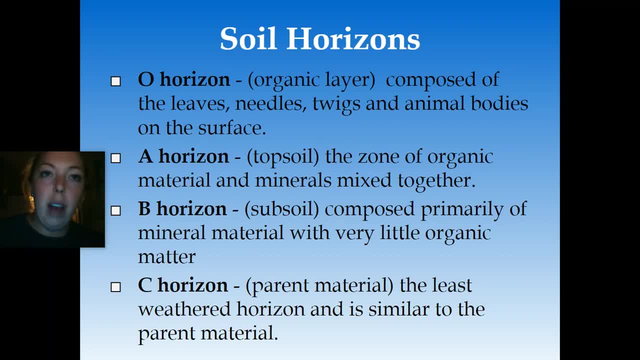 different nutrients in them. This all depends on those different factors. Okay, So at the surface of most soils is a layer of organic matter, right? Stuff that was once living, or is the waste from something that is living? right, This could be anything. 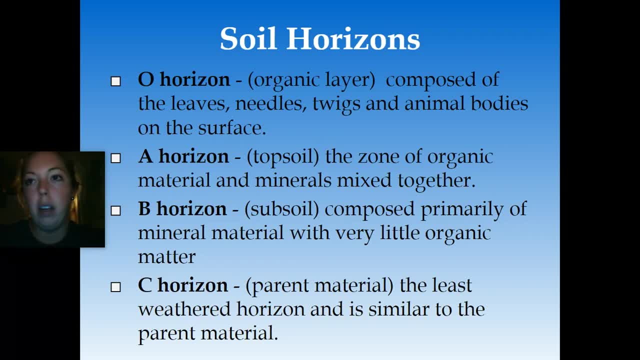 like tree needles, twigs, dead animal bodies in all different stages of decomposition. Okay, we call that top layer the O horizon. Okay, so that's right. here It's the organic layer. Alright, we also just call it the organic horizon: O horizon, organic horizon, right. 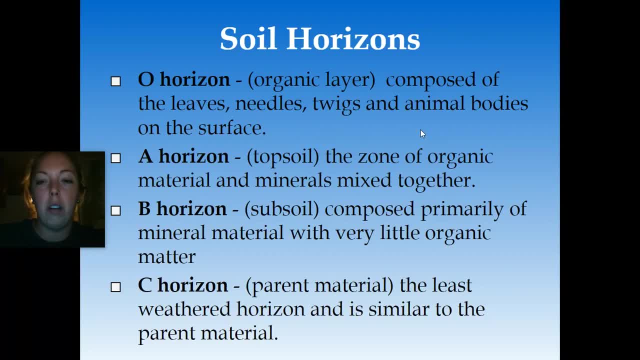 It's most pronounced in forests, soils and also in some grasslands. Okay, Because in forest we have lots of organic stuff building up on the ground and we have a larger O horizon, essentially. So, in a soil that's mixed either naturally or by human agricultural practices, right The top layer of the soil is the A horizon. 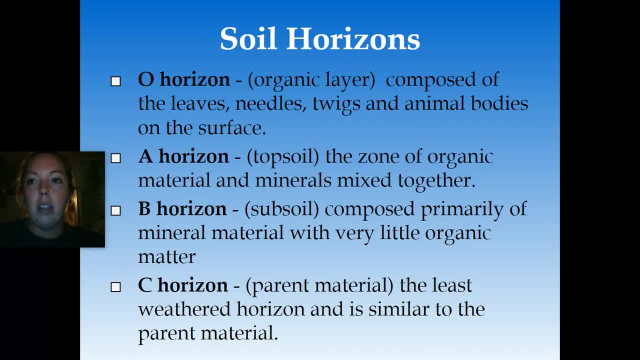 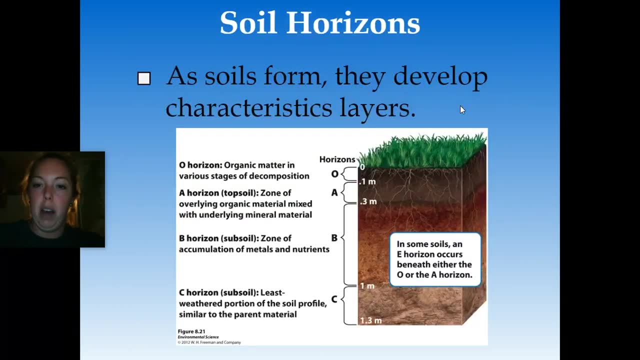 Okay, Another name for a horizon is just top soil, but the A horizon is a zone of organic material and minerals that have been mixed together. Okay, So if you're looking at the picture here- let me go back- You can see you've got O and A right there. All right, Because in most cases, 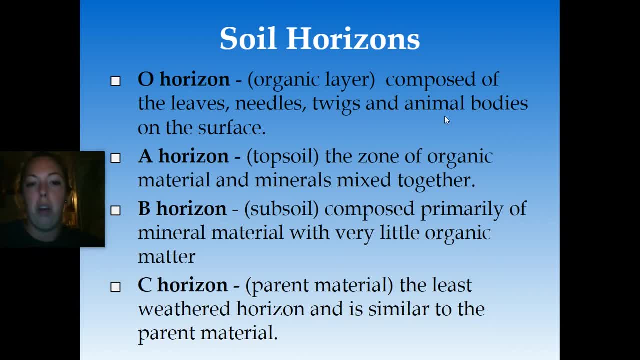 like where we're farming. the O horizon has just kind of been stripped away and we're left with the A horizon- the top soil on the top. Okay, One of the things you might see in your book when you're going through your reading guide is something about an E horizon. but don't worry. 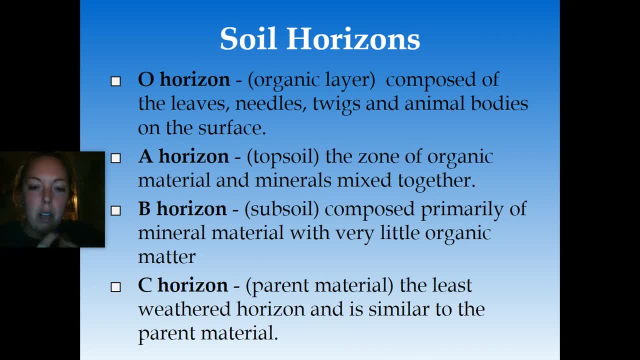 about that. We're not going to talk about it for our soil labs and other things. I just want you to know that. So if you're looking at your book and you're going through your reading guide, these four listed right here- O, A, B, C. Okay, But the layer beneath the A horizon is the B. 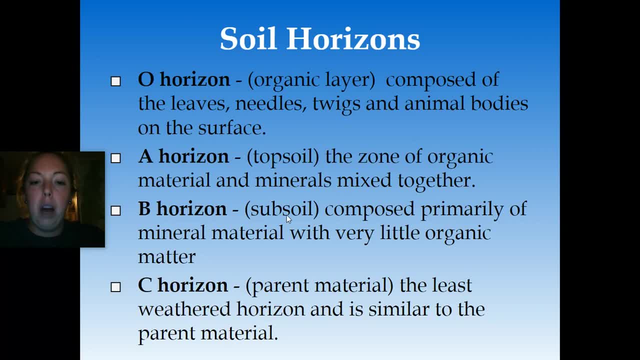 horizon. Okay, The B horizon is most commonly known as subsoil. All right, It's composed mostly of mineral material with very little organic material. So this is the first layer of soil that's getting most of its components from the earth instead of living things. Okay. 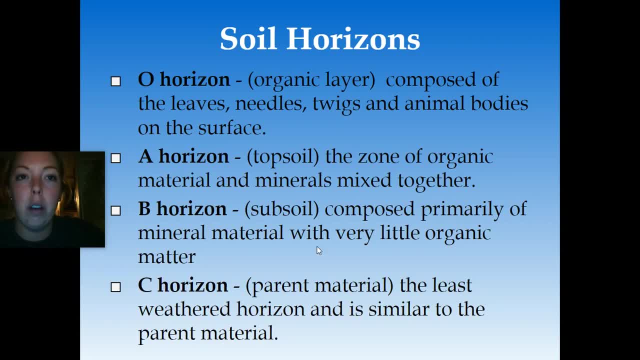 But if there are any nutrients present in the soil, they're going to be in that B horizon. Okay, The last thing, the last horizon that you need to know is the C horizon. So this is the least weathered soil horizon and it's always going to be underneath the B horizon. 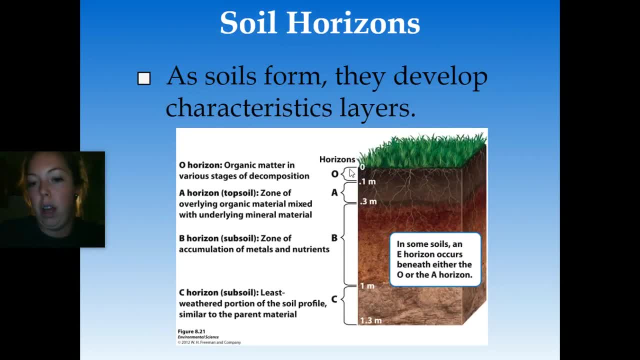 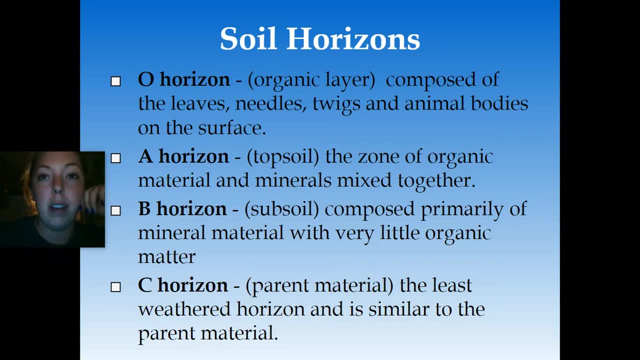 So let me go back to this picture again So you can see that O, A, B, C- easy peasy, right. The C horizon is similar to the parent material that the soil is originally from. Okay, But basically all of these horizons together have certain physical, chemical and biological. 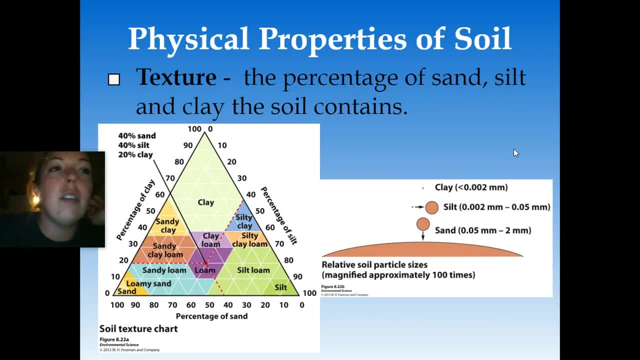 properties that they add to the soil. Oh, we're getting to the fun stuff, You guys, this is fun, So let's talk about physical properties of soil. All right, You are going to do a lab in class, or you've already started this lab, probably by the time you're watching this. that looks at the 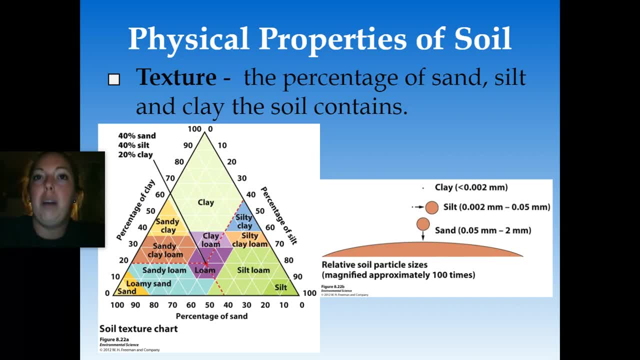 texture of soil. When we talk about soil in class, we're talking about two different things. We're talking about the physical properties and we're talking about the chemical properties. When we're talking about the physical properties of soil, we usually divide the mineral particles. 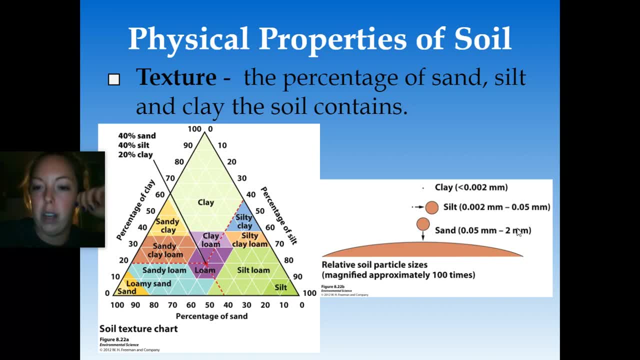 into different sizes. Okay, We call those sizes right here: sand, silt and clay. Okay, So I know you can see the measurement here, but sand are the largest types of particles that can make up soil. Okay, Silt is. 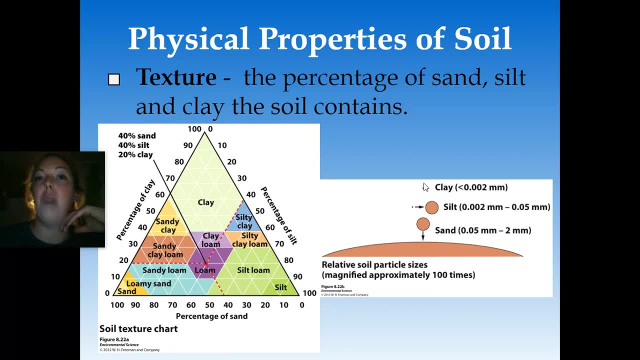 the next largest, and clay is going to be the smallest. So the way we determine the texture of a soil is based on the percentage of sand, silt and clay that it contains. All right, This is the lab that you're going to be doing, So we can put these percentages on a triangle that. 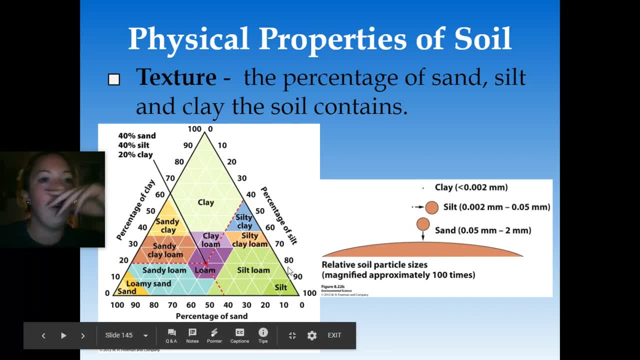 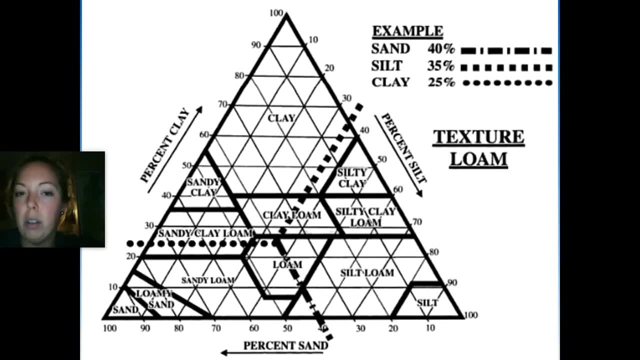 looks like this. So we're going to do a lab in class and we're going to do a lab in class and this looks like this. This is called a soil texture chart, or sometimes we call it a soil triangle, And we can use this to identify and compare soil types Anytime you're looking at the 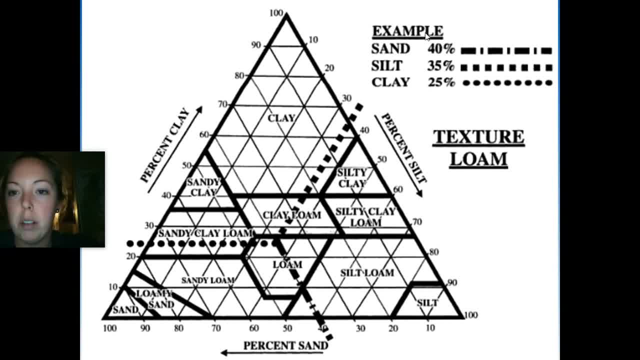 soil triangle. you're either going to be given these three numbers or the type of soil and not one of these numbers, or it'll be a situation like what you're doing in class, right? So you're doing a lab in the next couple of days of class where you are filling up your graduated cylinder with 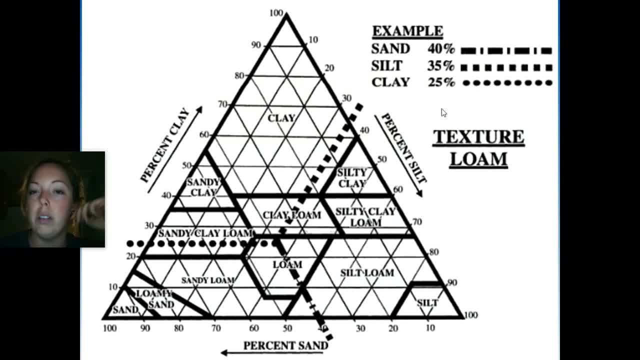 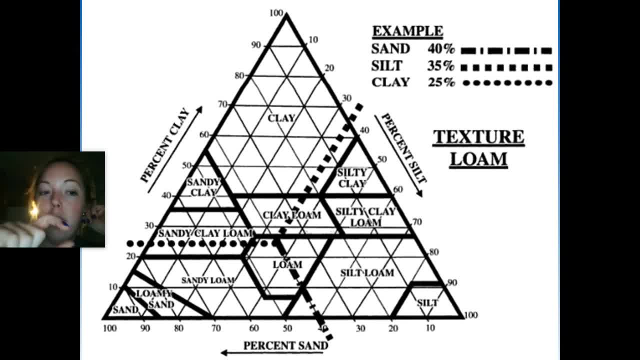 to be able to see the silt particles And on top of the silt you're going to see the clay, which is the smallest type of particle. So, based on that, you'll be able to measure exactly what percent is in your graduated cylinder, And we'll talk about that in class. I'll explain that again. But the 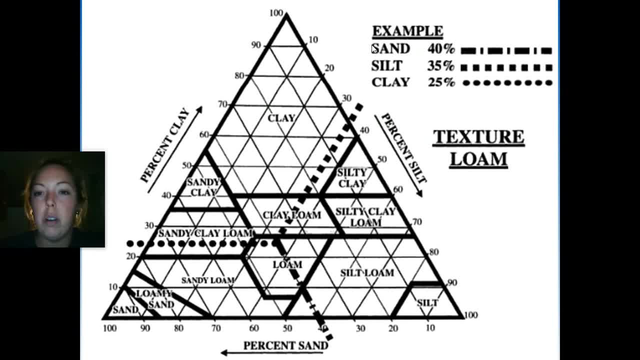 way it works when you're using this triangle here is you have to look at the numbers, Okay, So first let's look at sand, because in this example, it tells us that sand is 40%. So this is really really simple, But it's easy to get confused because there's three sides of the triangle. 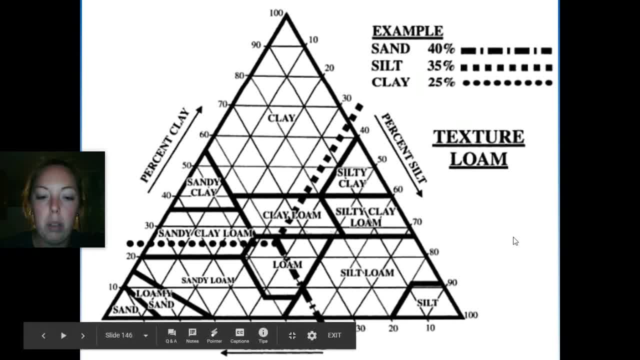 right, But what you do is you find the bottom- Oh, I hope this can go away- The bottom of the triangle here where it says sand. Okay, I'm going to try to. hopefully you can still see this. That's okay, But this is a percent sand, right? You have to go to the corner of the triangle where it starts. 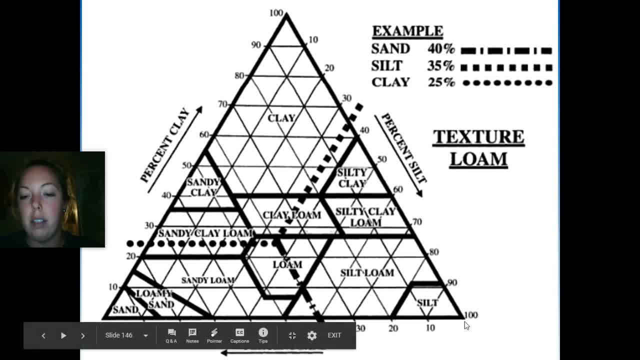 at zero, So you can see that it's a percent sand. And then you have to go to the bottom of the triangle where it says sand. Okay, So you can see over here, this is obviously zero and it's increasing 10,, 20,, 30. I know you can't see this, but 40 all the way up to 100. Okay, So what you do? 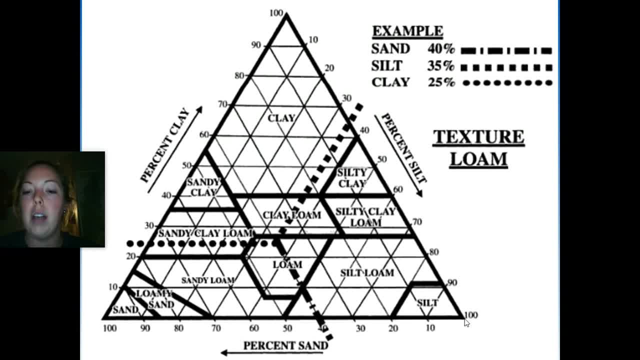 is you go to the corner where it starts at zero and then you're going to count over to whatever percent you have. So we have 40% sand, right? So we have to go over 10,, 20,, 30. This part right here. 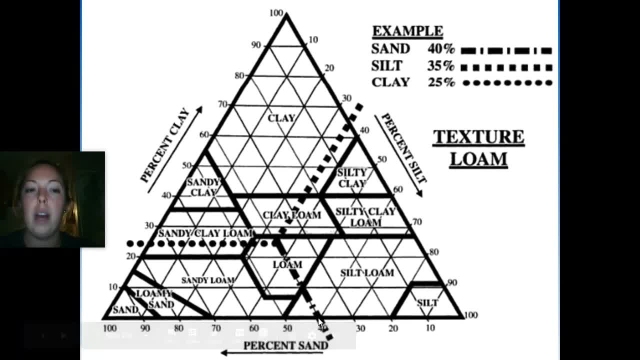 would be 40%. All right, So if you have this triangle in front of you, what you can do is you can just go to the corner of the triangle and you can see where the other ones go. Okay, So you want to essentially draw a line right here where it says 40%. So you're going straight up from that. 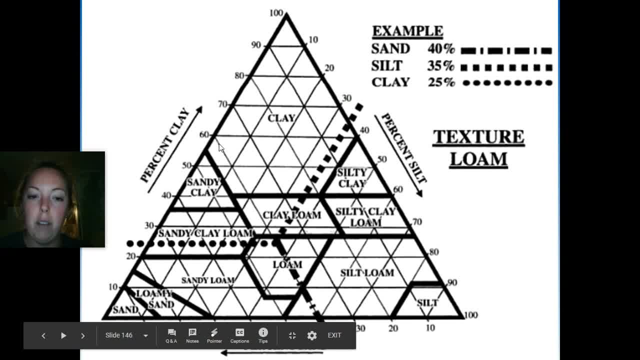 line. And that's the first number you have, But you just have to wait and see where the other ones go and where they intersect. Okay, So you've got sand at 40.. So let's look at the next one. The next one. 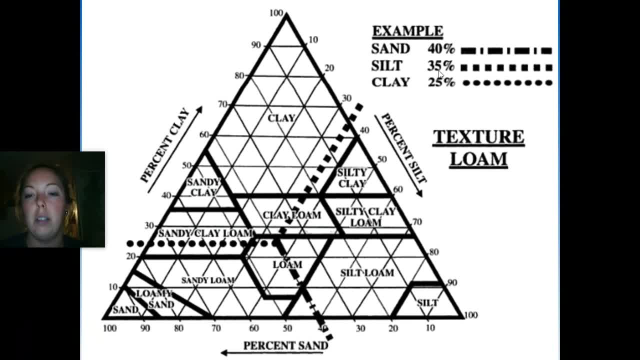 is silt. It says that our sample is 35% silt. So I need to find the side of the triangle that is for silt right. This is the percent silt. So I'm going to go to the corner of the triangle and I'm going to 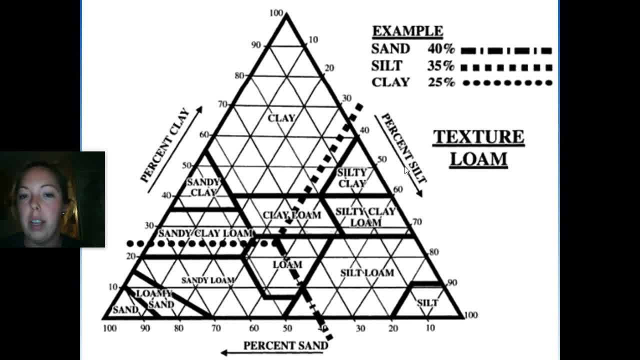 go to the percent silt side of the triangle. So, just like you did in the first one, you have to go up to zero. The zero is starting here And, as you can see, it's getting bigger. You have 10,, 20,, 30,. 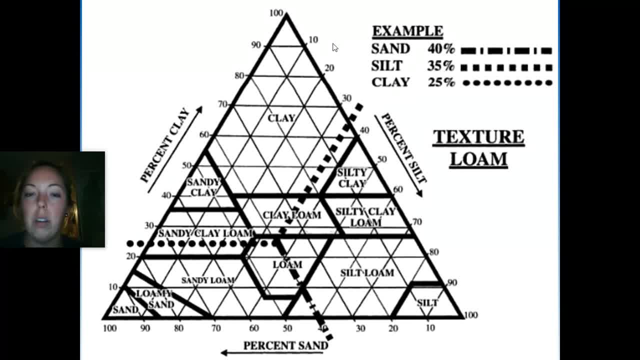 40, and so on. Okay, So we need to count up to 35. So you're going to start at zero. You got 10,, 20,, 30. Halfway through here is 35. So with your ruler, you can take it, lay it down. 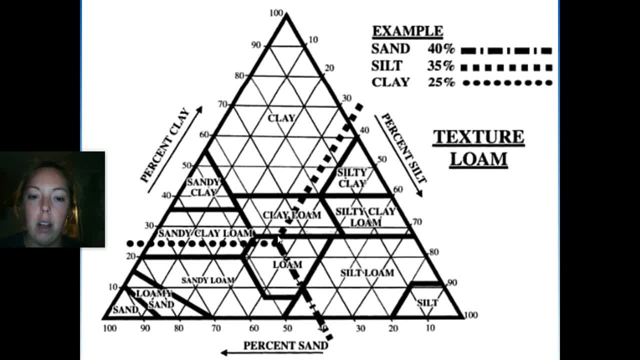 and you would draw a line directly all the way through the triangle, All the way to the end, if you want. But you can see it intersects here with your percent sand. So you can just kind of leave it at that if you want. Then the next thing you have to do is look. 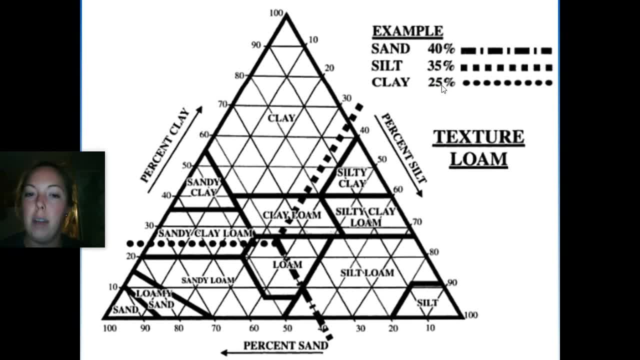 at the clay. The clay is 25%. So this is the last line we need to find in order to see where, on the triangle, our three lines intersect. Okay, So let's look at clay. This is a percent clay. Again, make sure you start from the bottom down here, at zero, instead of 100.. If you do it backwards, 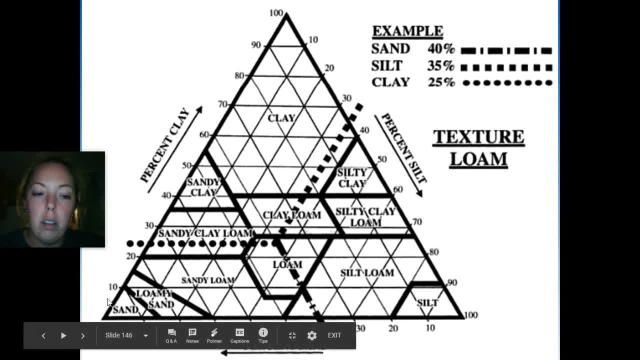 all of your lines are going to be messed up. So you go to zero. You got 10.. You got 20. And you have 25% clay, according to the example right there. So you have to draw a third line. all the 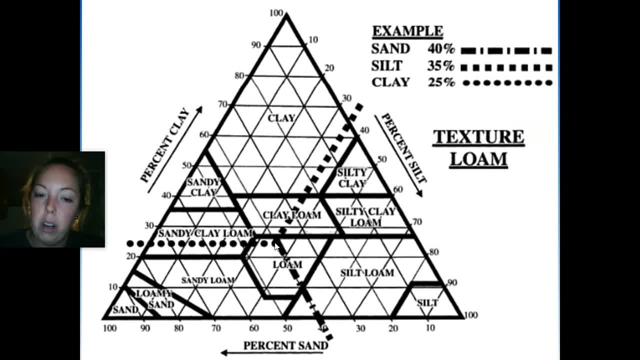 way across here if you want, Or you can stop where it intersects. But you're finding now that, when you look at these three lines, this is the point right here in the middle where it intersects. right, That's perfect. So all you need to do is find this point And then you're looking at the 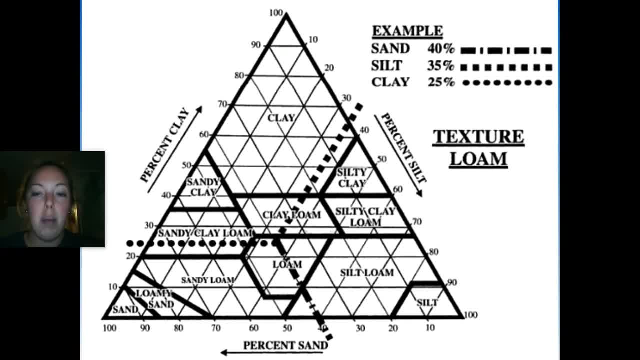 triangle to determine The name of the type of soil. Okay, So in this case- and it's really this easy, guys- it's falling under this category. So we would say that the texture of the soil is named loam. All right, If the three lines intersect somewhere over here, it'd be called silt loam If they. 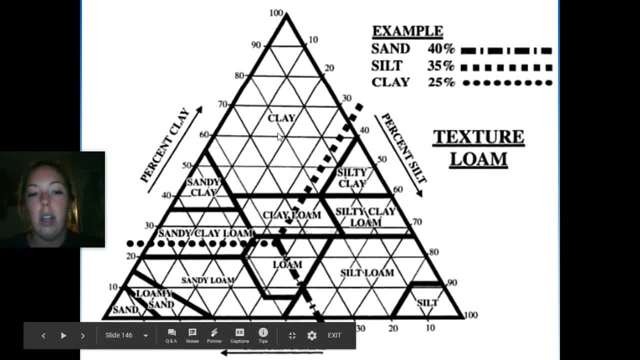 intersect down here. it'd be called silt, Okay, Or clay, or sandy clay, whatever, Okay. So it's going to be different for all the examples you have, But the samples that you do in class are going to be different because they're from all sorts of different places throughout Texas And 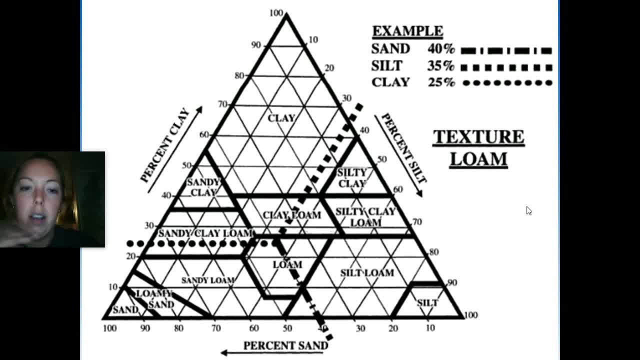 yeah, that'll be good because you'll get some experiences finding different types of soil, but definitely know how to use this soil triangle, because you will see this on quizzes and tests and stuff like that And the apes exam later on. probably Okay, So let's talk about the next. 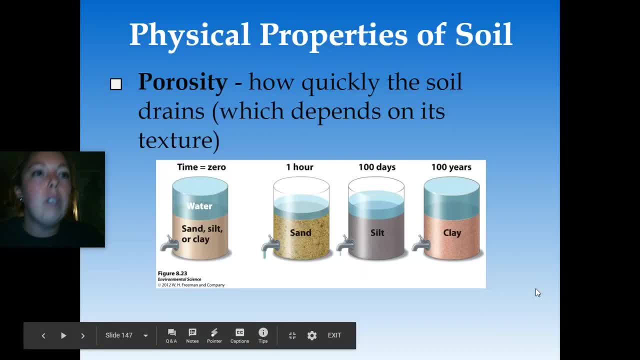 thing And I'll go over that in class again if y'all need some help. So let's talk about a couple things, some physical properties of soil. One of the things we'll talk about is porosity, And we actually talked about permeability and you guys did your permeability. 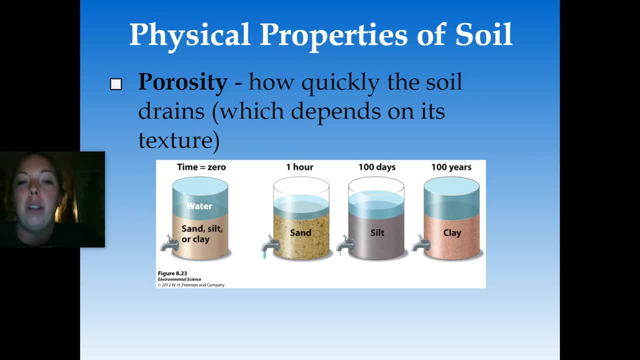 lab. but it's how quickly the soil drains. It completely depends on its texture. So, like we just discussed, sand is the largest type of particle, So water is going to flow through sand really quickly. This is just a diagram, for example. but if you were to pour water in the sand? 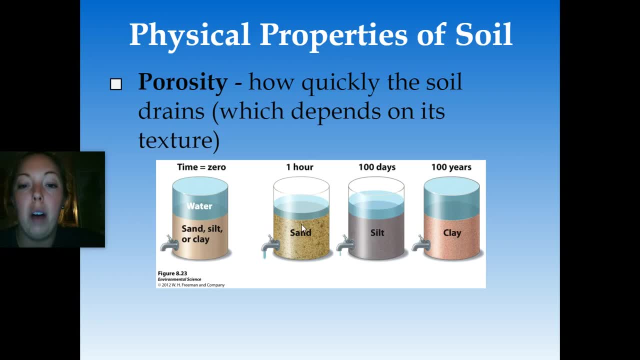 sample, sandy soil sample. it would drain out in about an hour. Silt is even smaller, So it's going to take longer, like a hundred days. Clay, if it's tiny enough, could take forever- Not forever, but this one says a hundred years. We're going to talk about it a lot more when we do our land use. 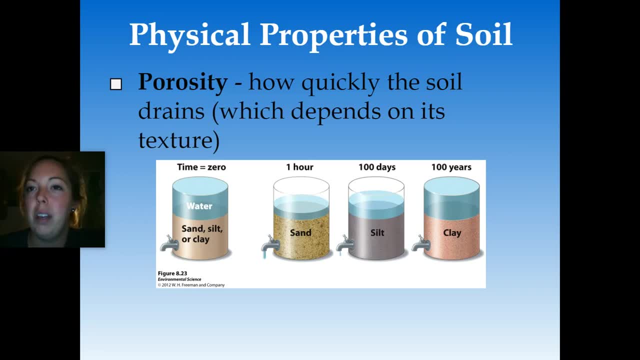 and agriculture unit. but the best combination of soil is something that's a mixture of sand, silt and clay. All right, Basically, if you have a mixture like that, there's going to be balance between water drainage and retention. right, Because, like we said in class, you don't want. 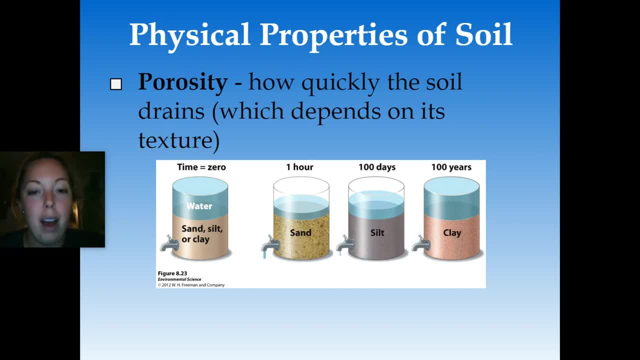 something that's really permeable, Where the water runs through the soil really fast or really slow. You want the middle there, right. When talking about the environment, our soil texture can have a strong influence on how the physical environment responds to environmental pollution. For example, the groundwater in Long. 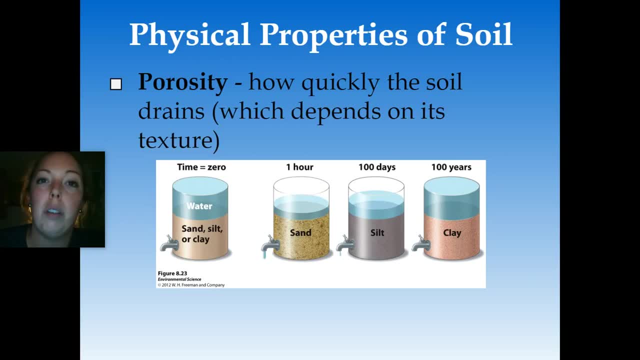 Island in New York has been contaminated by toxic chemicals that were discharged from local industries. Okay, So this is a big problem. One reason for the contamination was that Long Island was dominated by sandy soils, right? So if you have a mixture of sand, silt, clay and clay, 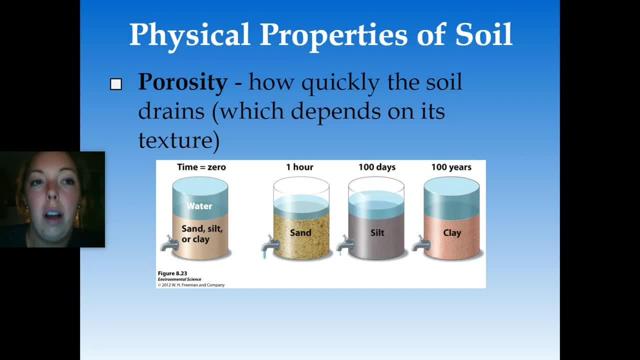 This is because the soil is very porous. We get so porous that the clay, silt and clay are very permeable and the surface water doesn't really filter through the soil. We are able to remove a lot of pollutants with the water, So a lot of these sandy soils. 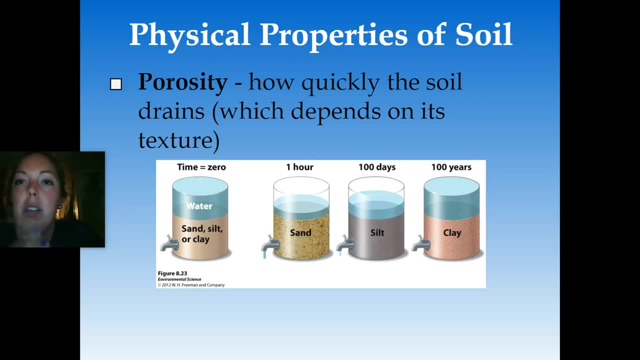 and this is really interesting, all right, but what we want to do is we want to remove a lot of the picture. So we're going to look at our water from the surface so that we have a look at that, But before we do that, I just want you to got the data again, right, Look? 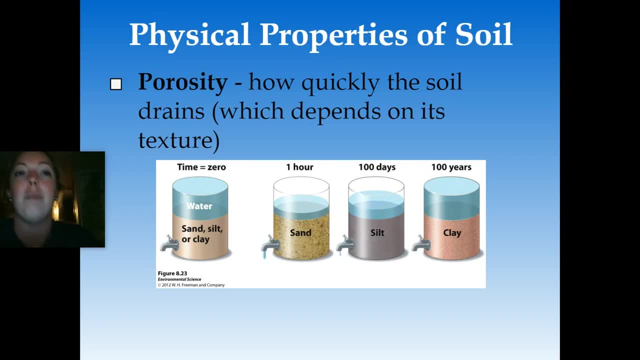 at our soil right now. This is a very, very strong polluted soil. We just get all these broken down by the sand. We're going to take a little bit of our soil out here and I'm just going to show you how we use this filter. Okay, All right. So these are our silt silt. 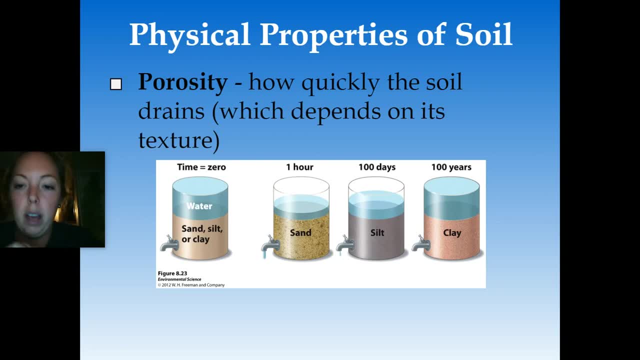 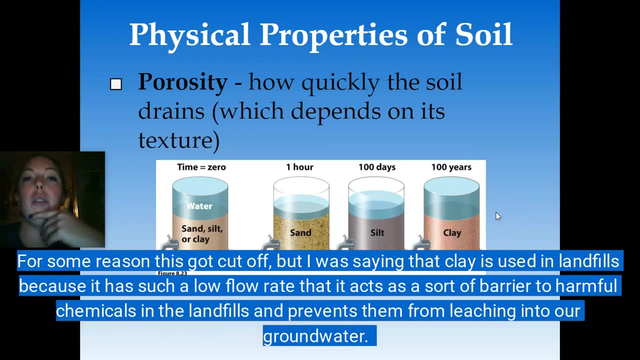 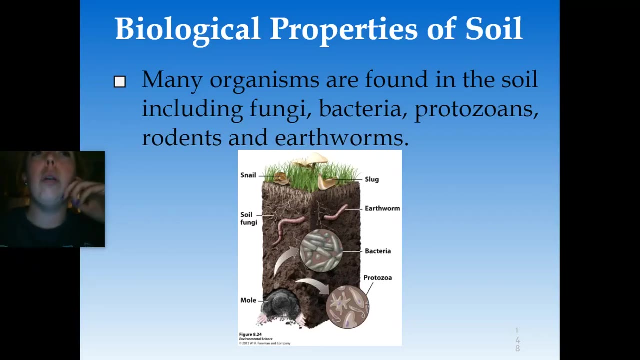 we get to our waste unit is clay okay, Because clay, as you can see here, is really really tiny particle size. wise, It takes forever for things to filter through it. Let's first talk about the biological properties of soil, all right, So, like we talked about a little bit earlier, there's a 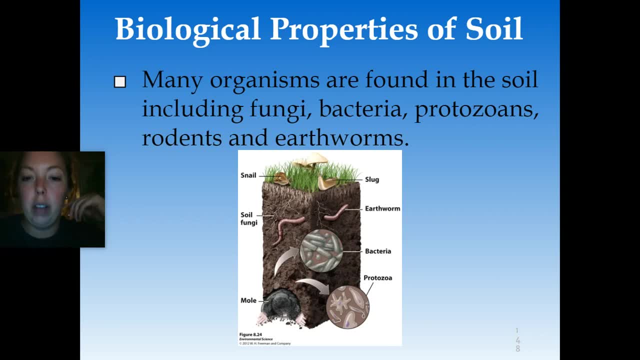 really diverse group of organisms that populate the soil. You guys can see some examples right. Three groups of organisms account for 80 to 90 percent of the biological activities in soils. okay, So these guys can include some of the things you guys see here. 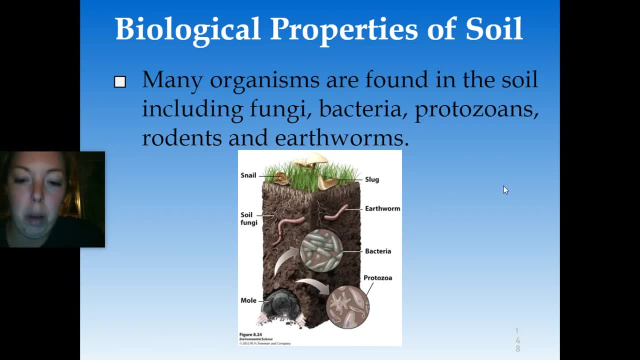 Fungi bacteria, protozoans, which, if you don't remember from biology, just means it's a single celled organism. Rodents and earthworms contribute to soil mixing and the breakdown of large organic matter into smaller pieces. Some soil organisms like snails, slugs, stuff like that. 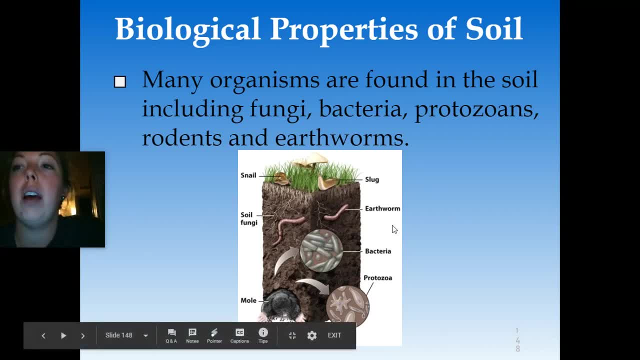 are herbivores, right, And they eat the plant roots as well as above ground parts of the plants, But the majority of soil organisms are detritivores, which means they consume plant and animal tissue and recycle the nutrients that they contain. So we'll talk about that when we get to. 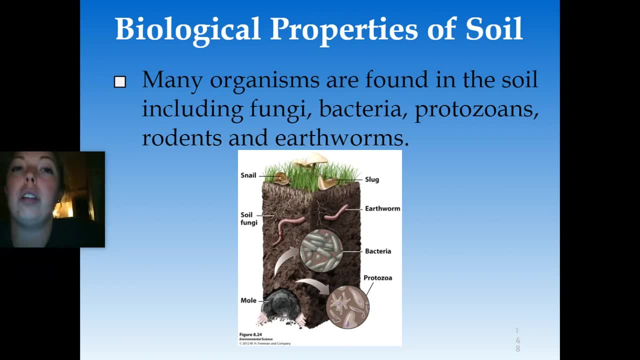 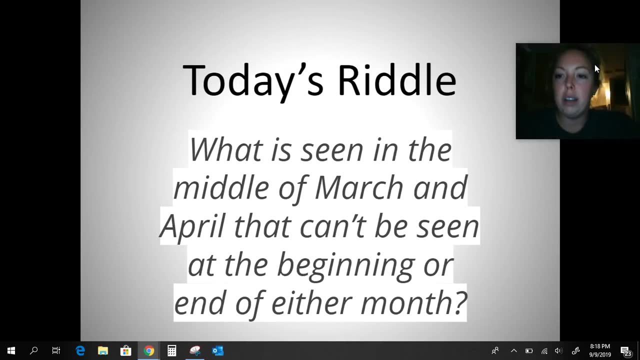 our next unit. But some soil bacteria also fix nitrogen, which is essential for plant growth. We're going to talk about all of that when we get to the nitrogen cycle. Okay, so let's call it good right there. Here's the 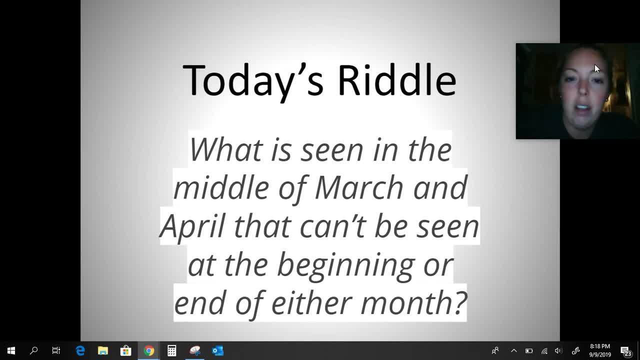 riddle for today. Let's see if you guys can get it and I'll tell you the answer in class. So what is seen in the middle of March and April that can't be seen at the beginning or the end of either month? Think about it and I will tell you the answer later. Do you guys want to see my dog? 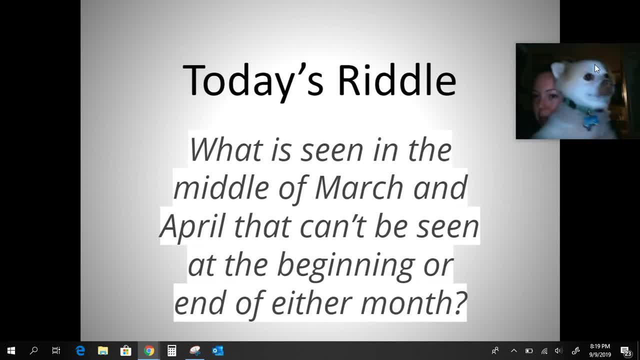 again. Goodbye my little apes friends. Kiba look at the camera. Kiba look at the camera. This is my dog, Isn't he cute? Oh my god, he looks so sad and miserable. He looks scared, Kiba.